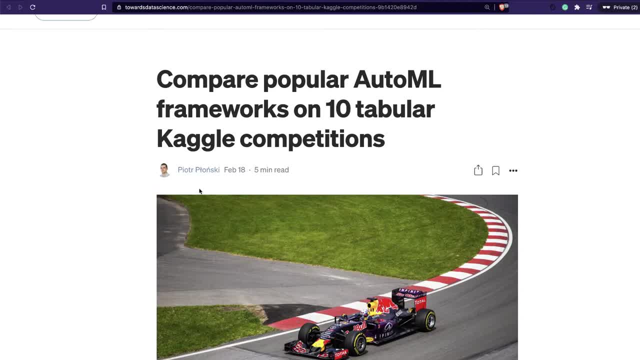 So what does 10 tabular Kaggle computations mean? Kaggle computations might have tabular data or, you know, not tabular data like computer vision or some media data. So what this author has done, PureAutor has done in this case- is: take 10 Kaggle computations. 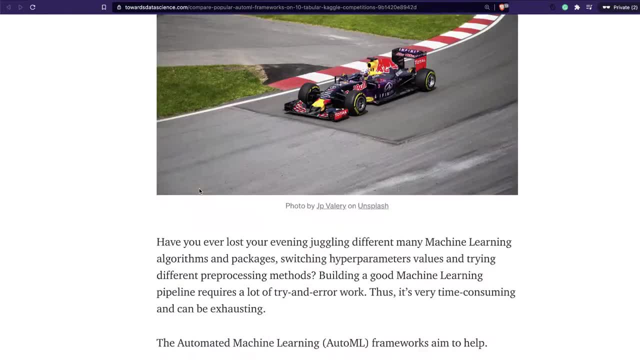 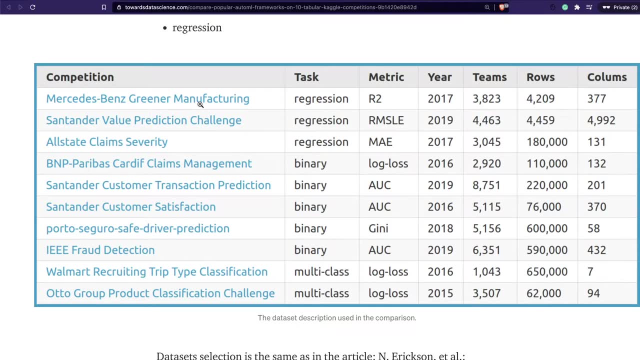 especially tabular computation, and compare it with these AutoML frameworks and what are the computations that he has picked up is something that you can see now. So the Mercedes Benz competition: so you can see that there is a Mercedes Benz manufacturing and the task is regression task, and then the Sandner value prediction challenge and task. 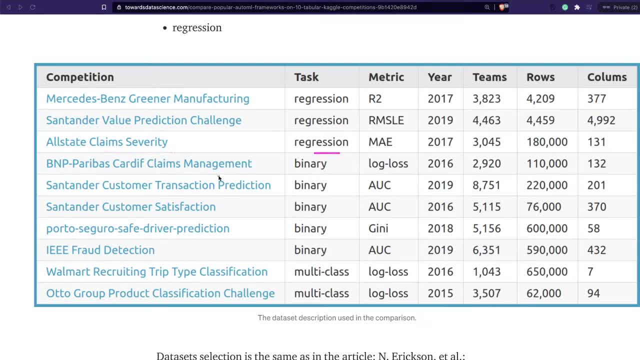 is regression, Allstate claims severity task is regression and you have got a bunch of binary task, which is a single class binary classification, and then you have got multi-class classification- Walmart recruiting and auto group product classification challenge, and you can also see the metrics that is used for evaluation of these computations. So whenever there is a 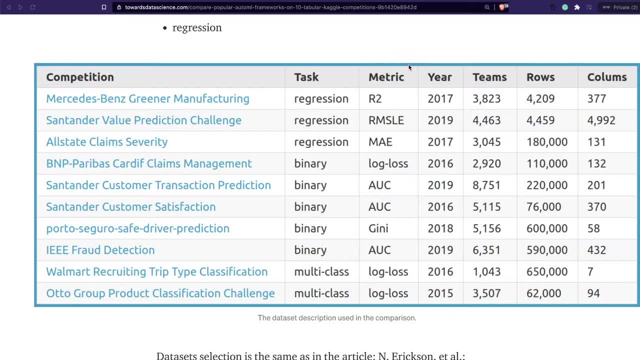 competition on Kaggle. so there is an evaluation that is going to happen, like you're going to get a final score, and that score is usually based on this metric, that is, that is announced upfront for competition. So people who are trying to do or win this competition, they would optimize their 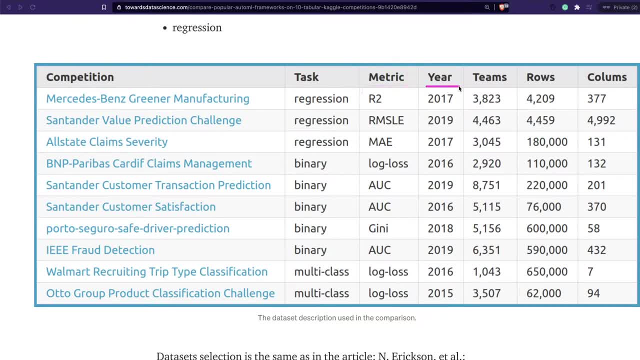 algorithm for this metric and when did this competition happen, how many teams participated, how many rows were there in the data? and then how many columns were there in the data? So this is the information. So we have 10. competition 1,, 2,, 3,, 4,, 5,, 6,, 7,, 8,, 9 and 10.. So we have 10. 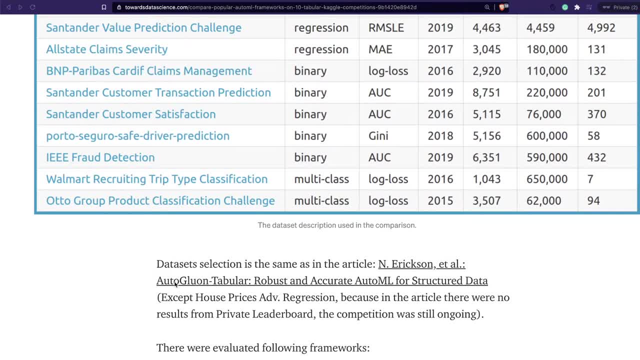 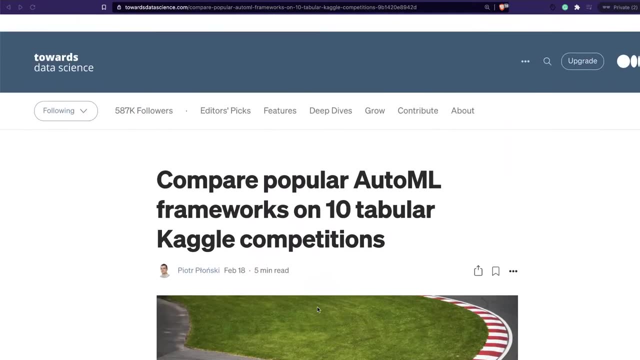 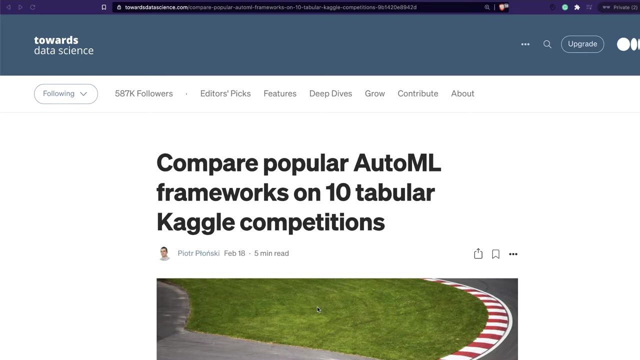 competition and these competition were picked up From this article, which is, which is actually you for auto glue on. So this was an article introducing auto glow and tabular, and those competitions have been picked up by Piotr to showcase the comparison of popular framework. and there is a small disclaimer that I would like to add. 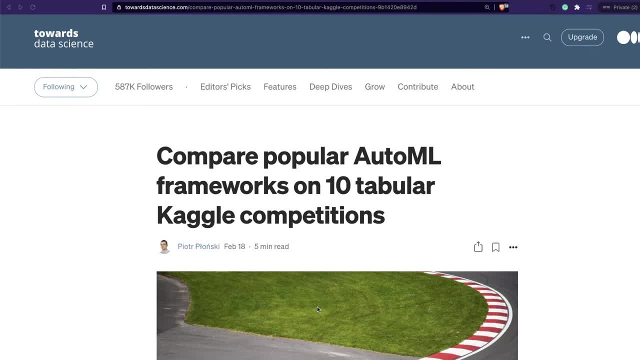 At the end of this video you might see that ML jar as an auto ML framework, that would come at the top for a lot of these competition like with good score. and ML jar is a package, a library, created by Piotr So so I'm not saying that there is something going on, but I would like to highlight 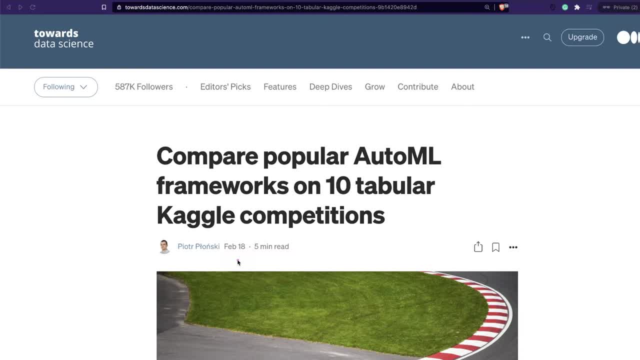 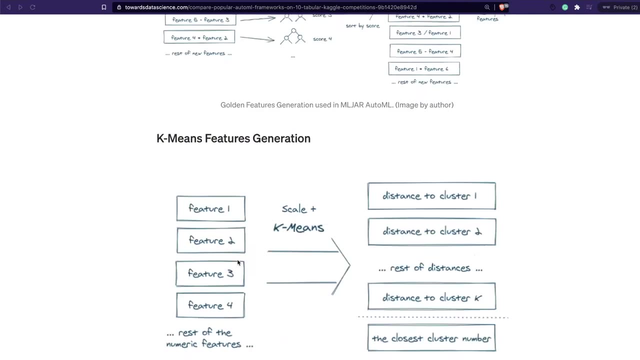 this as a fact because a lot of times, whenever we do this comparison, it's quite simple and easy for us to you know, miss these hidden details. Having this hidden detail would help us be skeptical always and then also explore further. Let's get started and then see what are the results look like. So we have 10 competition. 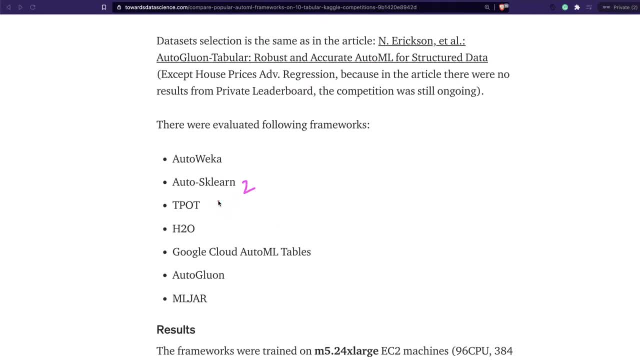 and then we have one, two, three, four, five and six and seven. So we have seven auto ML framework. So seven auto ML frameworks when compared against 10. competition from Kaggle and the author's reason for why he picked up Kaggle data set us actually. 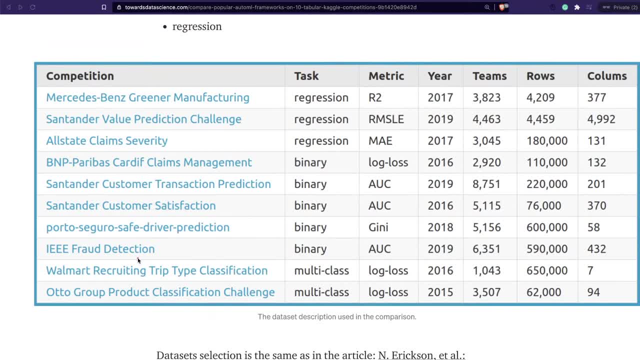 These are companies sponsoring a particular competition like this. This is like Mercedes Benz, This is like Santander. So these are actual companies sponsoring this competition and then people actually winning thousands and thousands of dollars as price money. So this would most likely replicate a real world problem. So that can actually tell us how auto ML can help in real world. 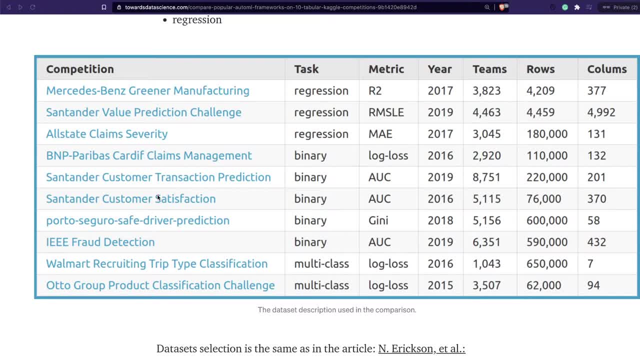 And the next reason is the comparison that that has been done here as part of this analysis is on the private leaderboard. So Kaggle usually has got- if you're familiar with Kaggle- for any competition. you have something called a public leaderboard and you have something called a. 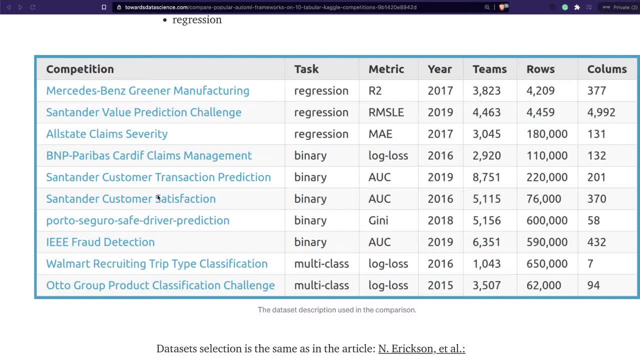 private leaderboard. Public leaderboard would try to evaluate your machine learning model on a very smaller subset of data. It wouldn't use the entire data and private leaderboard is the actual reflection of the entire data: how your model is performing well. how does it matter? 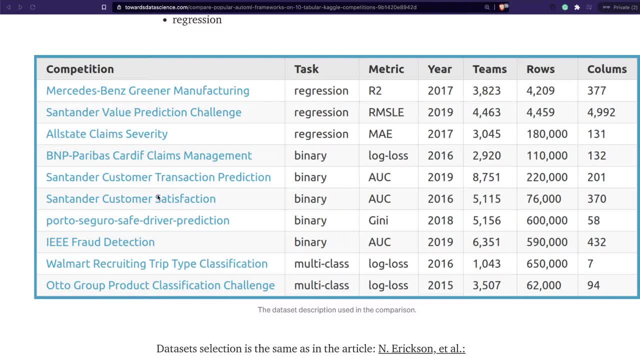 You could be optimizing your algorithm for public leaderboard very hard. it is entirely possible that you are actually overfitting And then when you go to private leaderboard, you are going to see a big shake up. That's what Kaggle call it- big shake up. 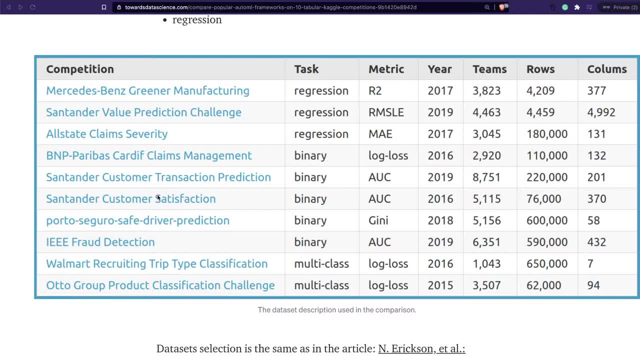 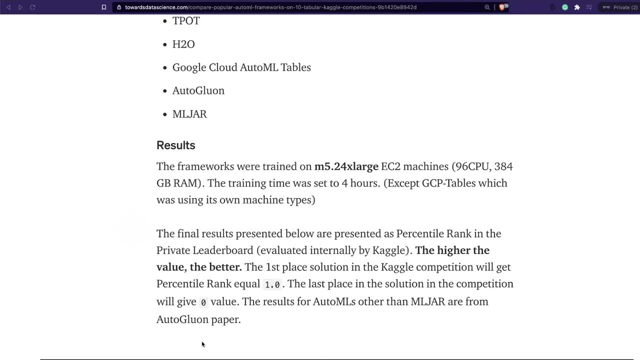 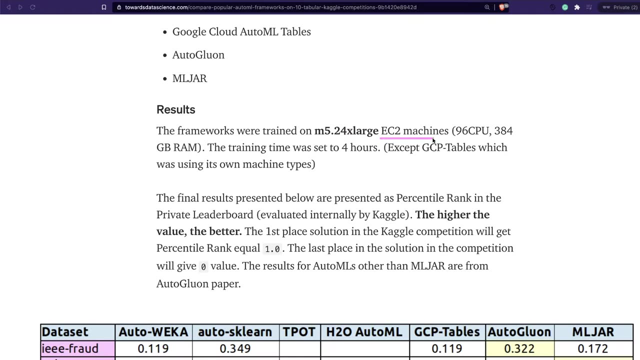 So that's why private leaderboard, which means the solution is also on the entire dataset. So that's another good thing why the author has used Kaggle. And regarding the machines, the computer that was used for this analysis is it was trained on Amazon EC2 machines. 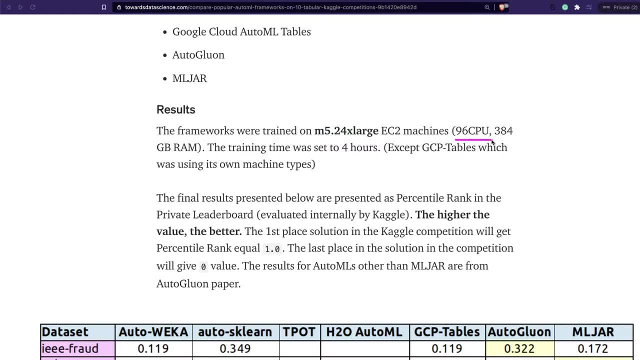 2x large machines, 96 CPU, 384 GB RAM- You can assume that the amount of computation power that is required for this kind of piece. Then training time was set to four hours. So this data is applicable, except for GCP tables, because they're using their own machine type and 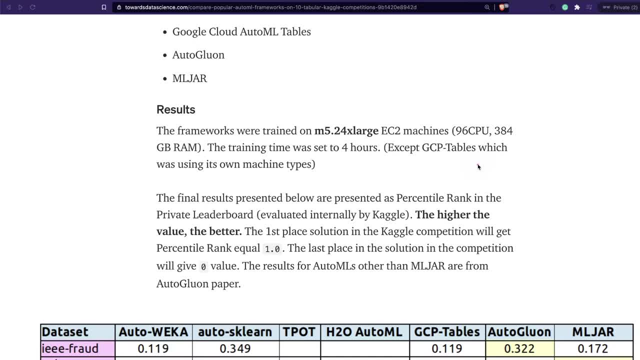 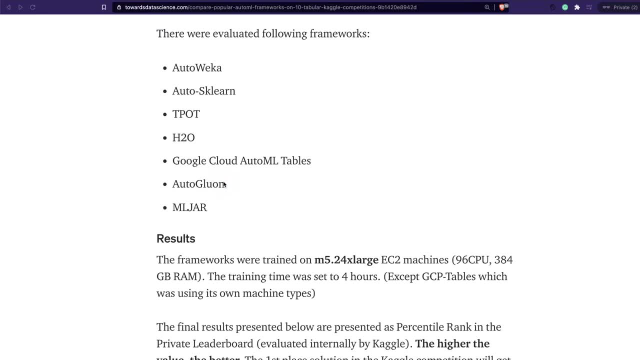 then you don't have control on the machine because everything else is like an open source package, The Python package. you can just install it and then use it, except Google Cloud AutoML table, which is part of your GCP package, or you need to have GCP credits for you to do it. So, given that this is the situation, 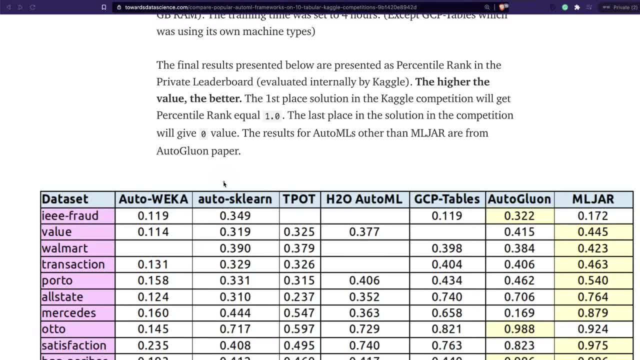 this is how the final result is going to look like, and how do you read this result? So the score that you see is actually a percentile rank score. So what does it mean? It means if you imagine there are thousand people who participated in a competition. 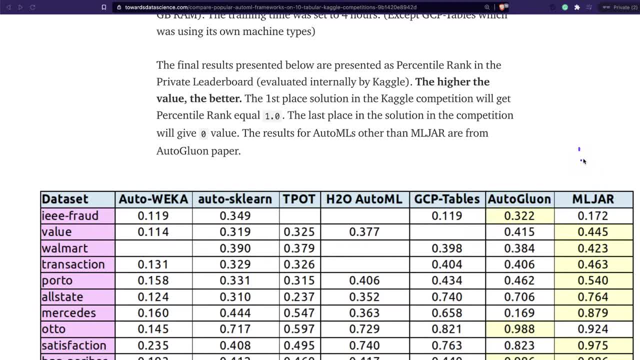 the first rank, first rank: whoever gets the highest score, they are the ones who get the highest score. So this is like 1.0, 1.0 as a score, 1.0 as a score. that is like the best solution and that's. 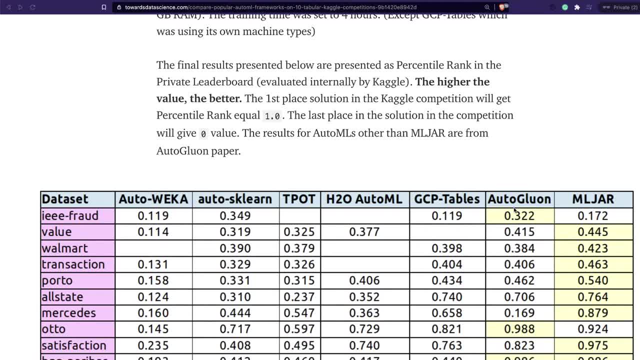 like the first rank and whoever has the worst solution, their rank is zero. So anything in between you can see, from best to worst, from like one to zero, which means higher the value of the score is better. So whenever you see a higher score, 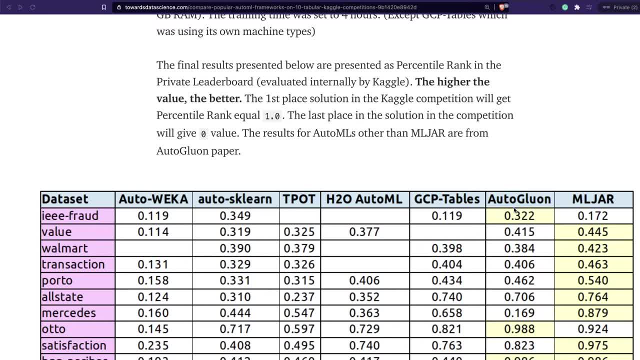 then the value is better And, if you like that, that that is what we are going to see here. So how, how this is going to be. So that's what we are going to see here. So how, how this is going to be. 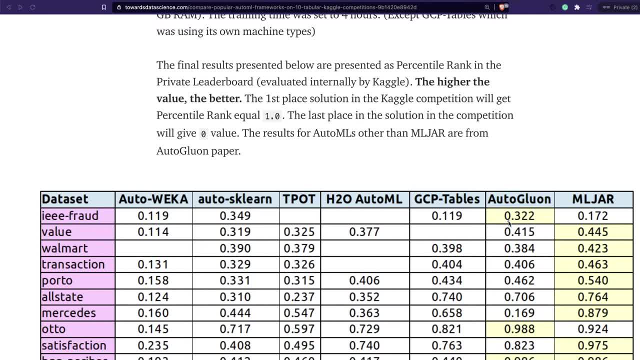 So that's what we are going to see here. So that's what we are going to see here. So the author has tried to highlight the best score, but you can have a look at it, you know yourself. So higher the score is better and it is from zero to one And it is what you are seeing is 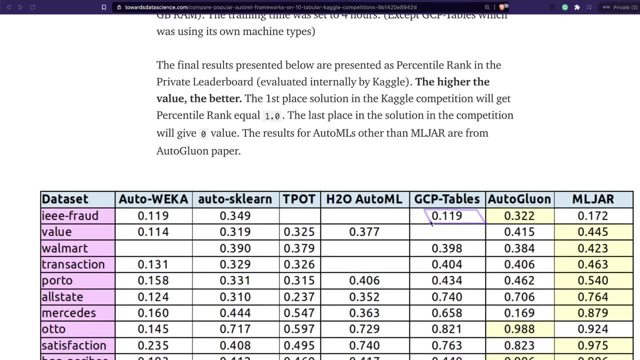 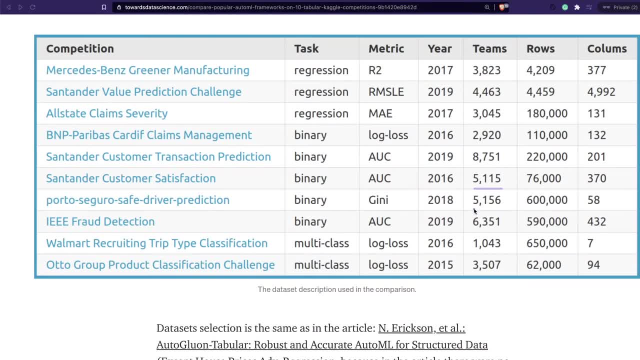 a percentile score of a given competition. So like you cannot compare two different competition now because the number of participants for different competition would change. You're like: this is like 5,000 people had participated. There's like 8,000 people had. 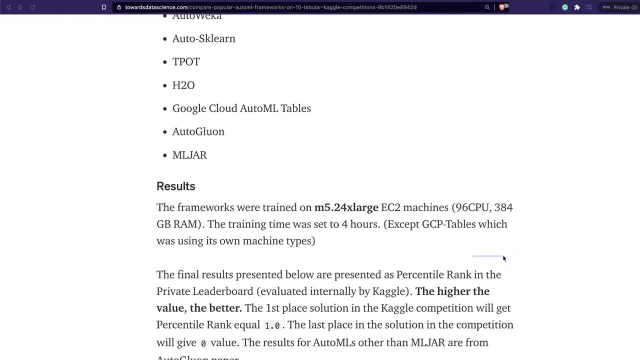 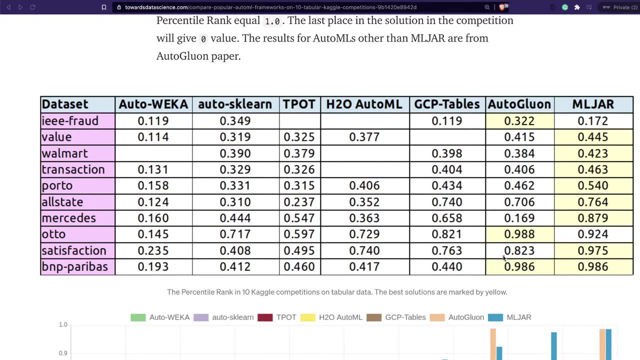 participated. There's just 1000 people had participated. So this, this would change. But what, what? the fact of what doesn't change is how better this particular AutoML package has done in a given competition. So we have got 10 competition, seven AutoML packages. 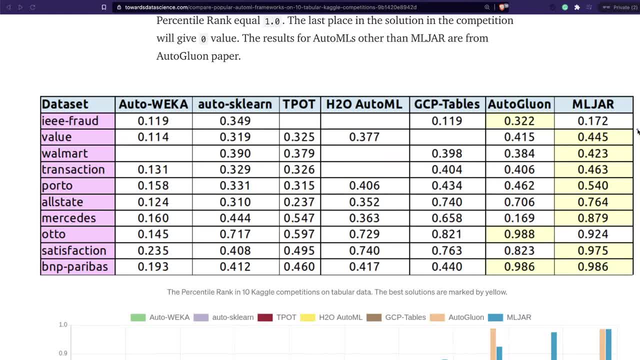 And if you actually see the MLjar has been a consistent performance in a lot of these competitions, which is a good thing You can see. like for these competitions, like the ones at the bottom here, you can actually see the AutoML solution has got like more than like 90- 90th percentage, which which 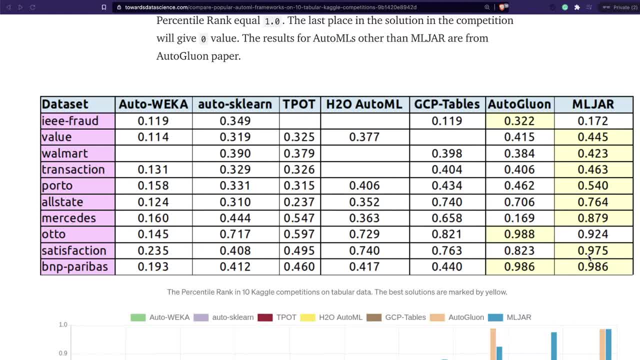 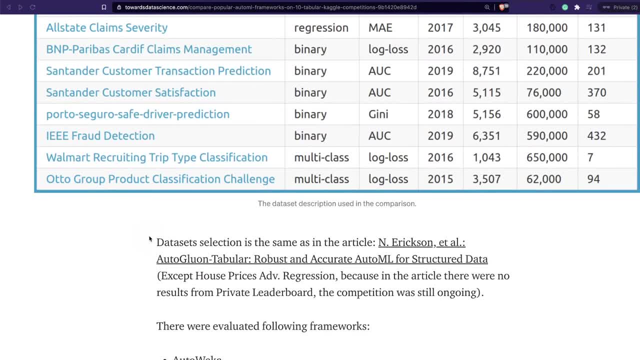 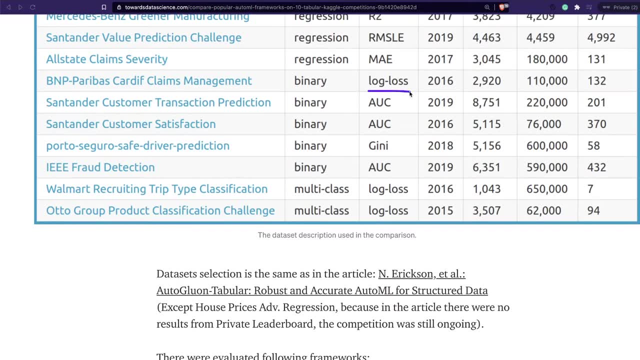 which. what does it mean? it means these AutoML solutions, for example. let's, let's take BNB Paribas- okay, the competition that we just saw here, which is BNB Paribas Cardiff claims management. it's a binary classification problem and in the metric evaluation metric was log loss. so in this, 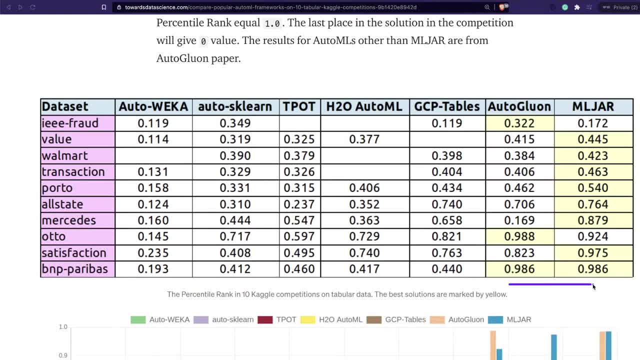 competition if you had used only AutoML solution. right, you have used only AutoML solution, either auto glue-on or ML jar. you are placed in the top 90th. sorry, top two percentile. so what does it mean? it means you would have easily hit a silver medal, most likely, I assume in this case you would. 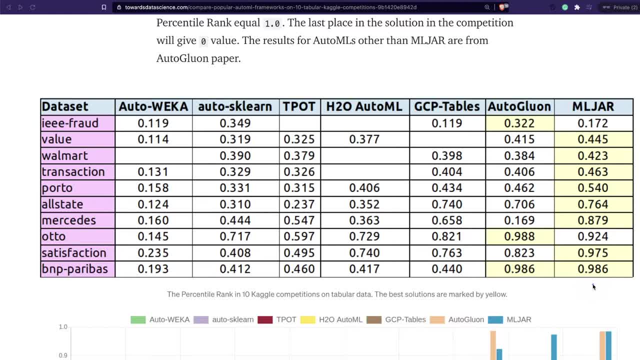 have easily got a silver medal on Kaggle for this particular competition if you had just simply used AutoML- you don't have to do, you know anything else yourself, they're simply using AutoML solution- would have gained you a silver medal in this competition and probably in all these other competitions as well. it would have got. 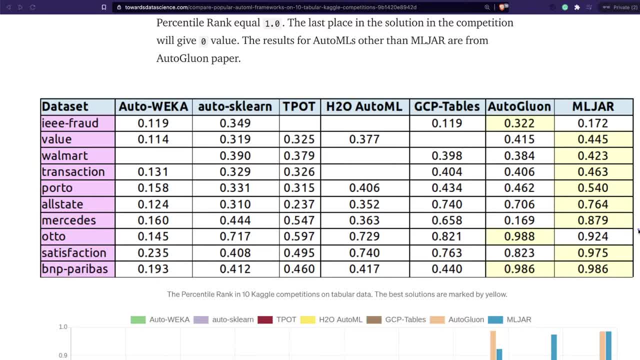 you at least at least a bronze medal, which is, I think, usually awarded for top 5% or something around like that. so what, or what does it mean for AutoML fans like me? one, AutoML actually works, works a lot. and when you compare it with when 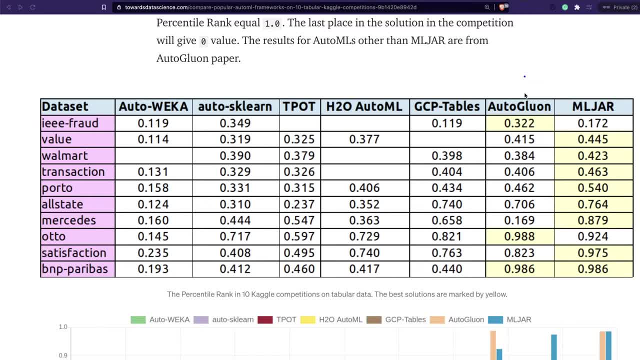 you compare it with the different solution, you can actually see auto glue on has been a consistent performer for a lot of this competition and, like the winner that you see in this case is ML jar. but what I would suggest is, like I have huge respect for the author, Piotr, who has put it together. no offense for 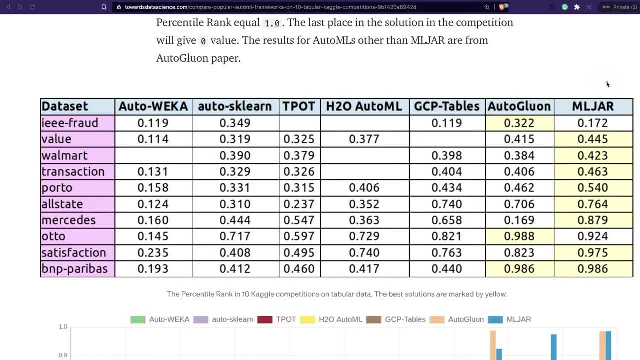 this analysis. I I highly respect you for this analysis. I highly respect you for this analysis. I highly respect this analysis. but still, what I would say is that the way every AutoML algorithm works is different. something would require a lot of computation power. for example, not every day you are going to have a 300 GB machine for you to run. 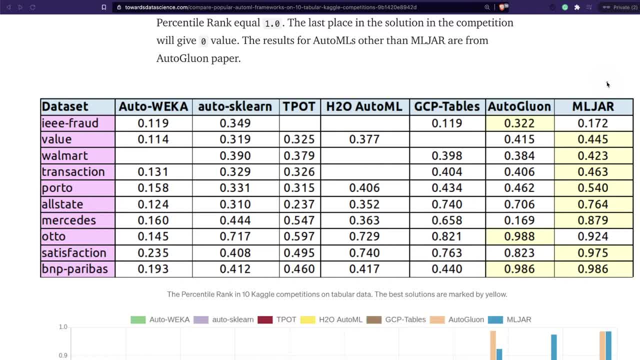 AutoML forever. so there are instances where- like for example, to give you a sense- h2o can give you a better result. like in my personal life, I have one hackathon just using simple h2o. I'm not saying that is the best, I'm just saying 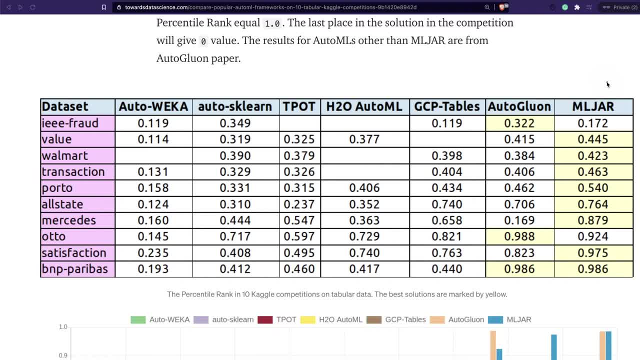 that I'm not saying that is the best. I'm just saying that I'm not saying that you need to pick the AutoML solution. not just be purely based on the highest score that you can get, but based on a lot other factors like how much computation power is required, how much information this AutoML is going to give. 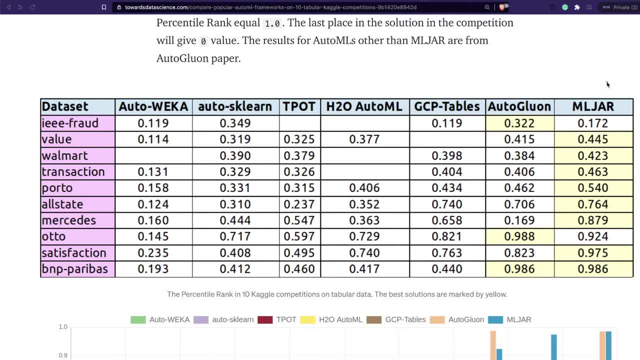 you regarding what is going on behind it. so all these things, so overall ML jar has done a really good job, followed by AutoGlue, and then you can also look at other solutions as well, like, for example, if you already have a GCP, ecosystem in GCP is really good, and and you can also look at other solutions as well, like, for example, if you already have a GCP ecosystem and GCP is really good, and I'm 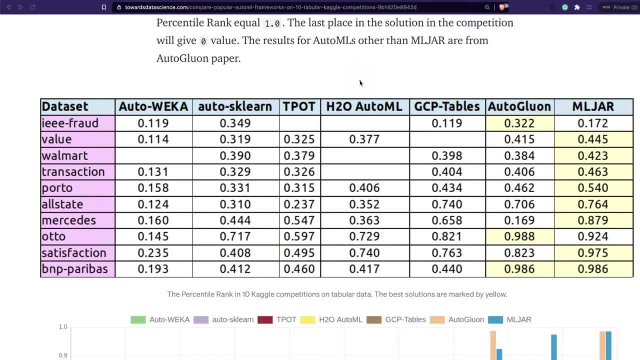 and if you, if you want, if you want a solution that can be easily productionized, h2o is good because h2o can give you the jar files that you can put it in your java java production system so that moving, like the model to production, is quite easy. Auto waker: I'm not sure if it is such a. 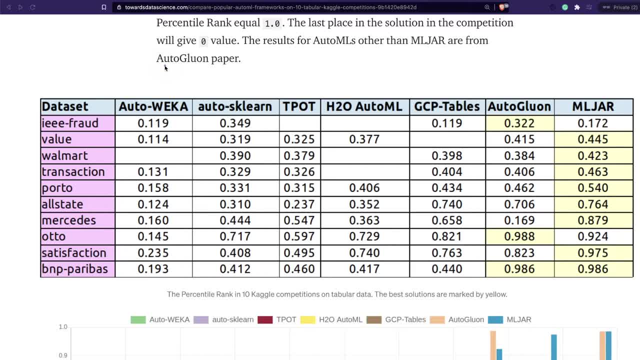 popular AutoML framework, like maybe it was just just added. Auto scikit-learn is a popular AutoML framework, like maybe it was just just added. Auto scikit-learn is a another simple package, but there are like other packages as well, like Auto, another simple package, but there are like other packages as well, like Auto. 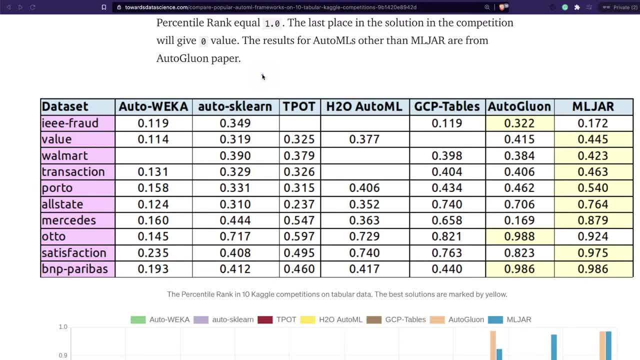 Keras, a lot of other packages that could really give competition to this Keras, a lot of other packages that could really give competition to this thing. AutoGlue one is actually definitely a promising package and a thing: AutoGlue one is actually definitely a promising package and a 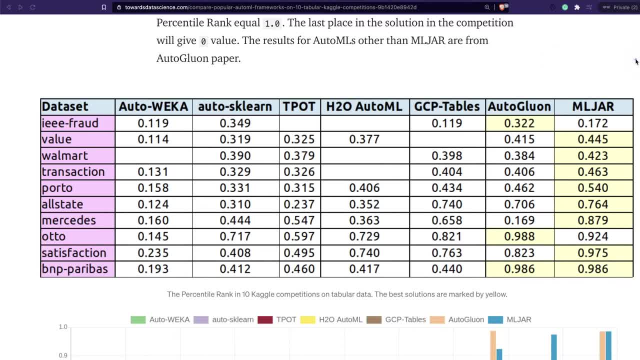 Mel jar is from this course. we can actually see ML jar and AutoGlue one are. Mel jar is from this course. we can actually see ML jar and AutoGlue one are very close and a Mel jar is actually a very good contentor for AutoML solution. 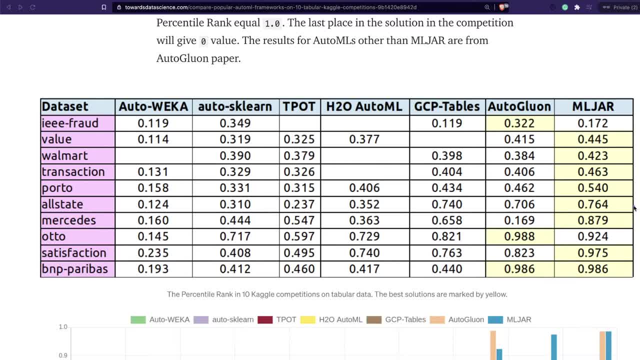 very close, and a Mel jar is actually a very good contentor for AutoML solution. so that's what this table actually tells us. but what I'm most interested is looking at these competition. uh, auto ml is really a very good way to start your baseline if you are going to participate in cattle competition or if you want to build a machine. 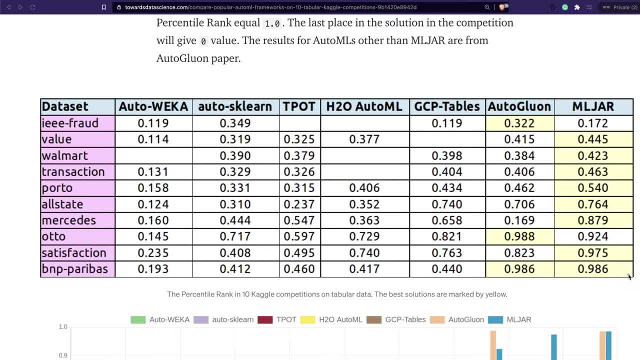 learning solution for your own organization. auto ml is definitely a very good way to start with the baseline um and um, like then you can pick the best model and then you can start tweaking it. but, um, but, instead of you doing all the heavy lifting, you know to start with like a lot of detail. 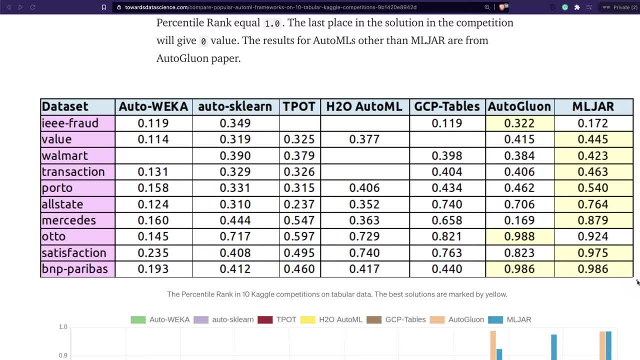 scientists. if you see, there they usually have a pattern right. somebody would start with a logistic regression or somebody would start with a random forest with a baseline uh parameter and then they would start uh optimizing their hyper parameters and then they would, you know, improve their score and probably move on to different algorithms. but having an auto ml uh framework can really help. 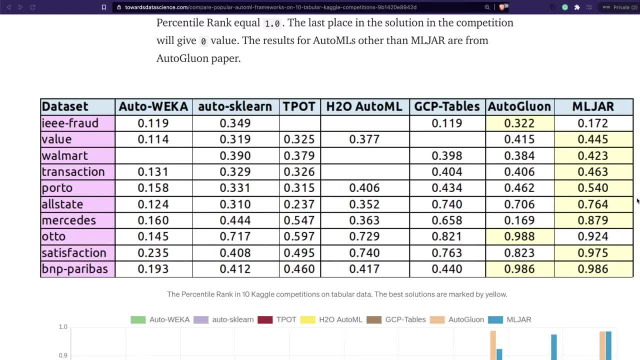 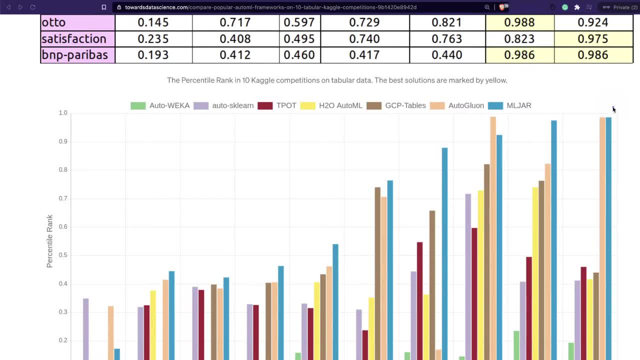 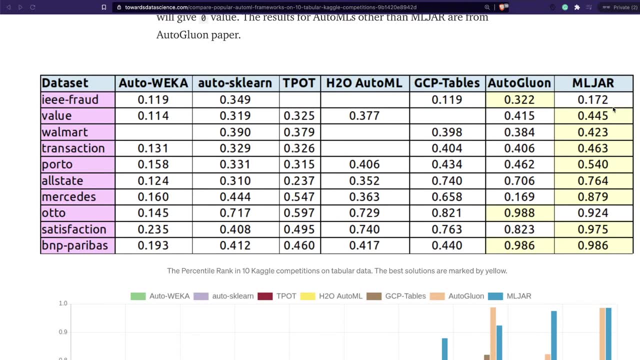 and that is, that is what these scores really indicate, and these scores are really visualized here. you can see, uh, blue color, ml jar being quite at the top for a lot of these competition. once again, um, this, this video has nothing to do with ml jar, or it's not being. 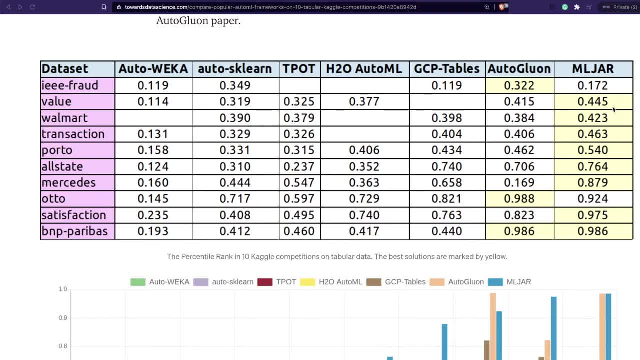 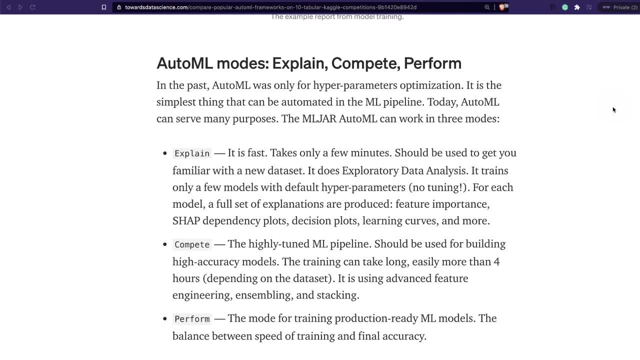 sponsored by ml jar or anything but ml jar really, really looks like a nice um auto ml package that you should check it out and that that probably takes us to the end of this video. so i want to wind up this video, you know, uh, giving you some. 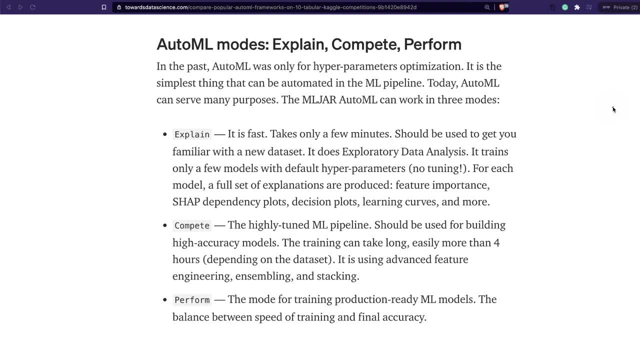 information about, or my experience about, auto ml. first, you might wonder: why do you need auto ml? let's see, you are a data scientist, uh, or you are a machine learning engineer. why do you need auto ml, right? um see, uh, according to me, if you ask me, uh as a data scientist, i would uh be more interested. 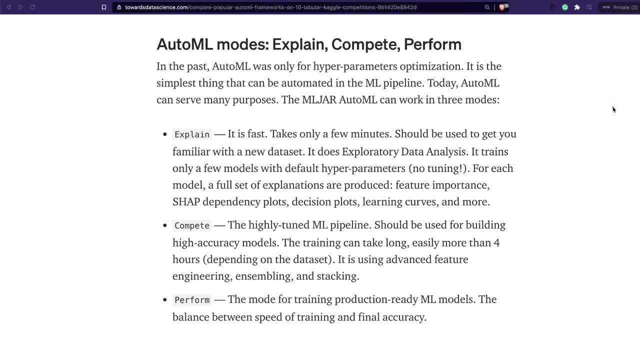 in solving the problem that i'm trying to solve, rather than, you know, like, uh, doing a lot of trial and error. so what auto ml does is, for me, is it actually takes care of the trial and error process, builds like, let's say, like 100 models, 150 models to 100, 000 model, 2000 model, like how many number? 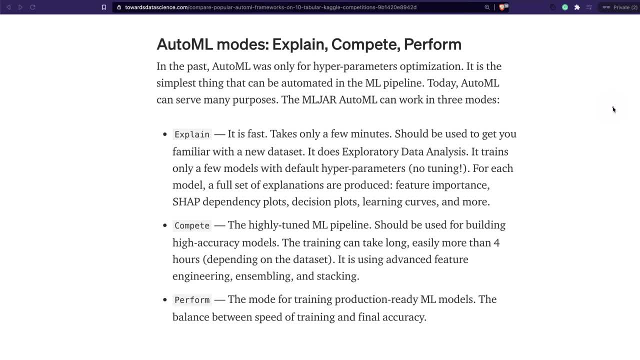 it is. and then it is going to tell me, uh, uh, this, these are like the top five best models. and now, based on my organization situation, my necessity, um, what is better for my company or what is better for my development environment? i'm going to pick something from that and then 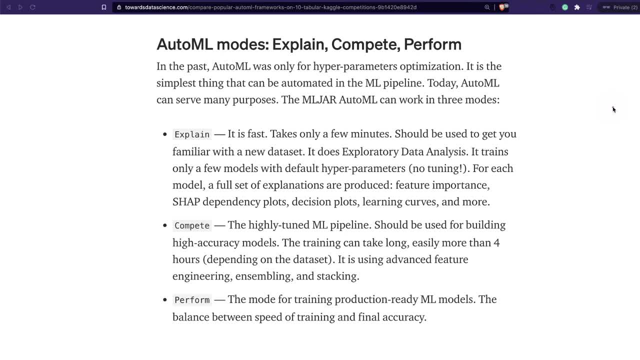 i can start building on top of it. so that is the biggest advantage auto ml has got. biggest advantages. not everyone um is actually um, you know, like um, let's say, a high-end data scientist like some, somebody like you know, like forex gaggle grandmaster or something. 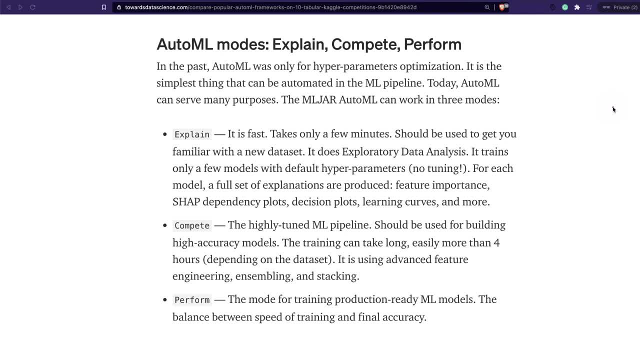 so if you do not have a very strong um data science team, let us say, but you still have problems and you want to solve them, maybe like you've got software engineers, maybe like you have got a bunch of people from devops who wants to try this thing. so what do you do now? like you, you don't. 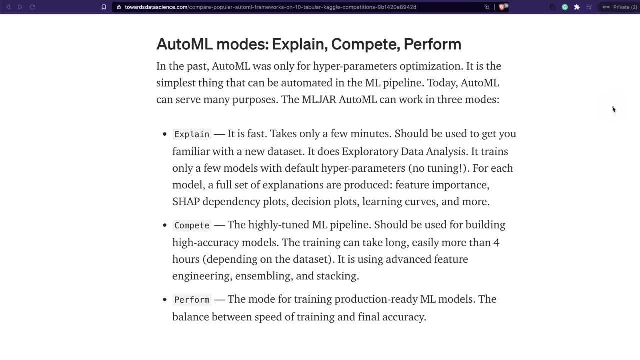 understand all these stuff, but you don't, you cannot, you know, send them to do two years graduation and data science and then come back, and that is really where auto ml is again really, really helpful, because all if you want is a baseline model that gives a decent accuracy. 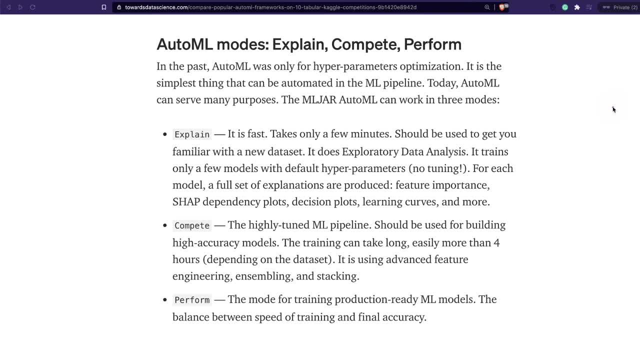 like we. we just saw, uh, for a few competition it was. it was even the top five percentile, top two percent, right rank based on the evaluation metric. so in that case, uh, your auto ml can give a very and um, your software engineer can build it, your devops a person can build it. and then third, 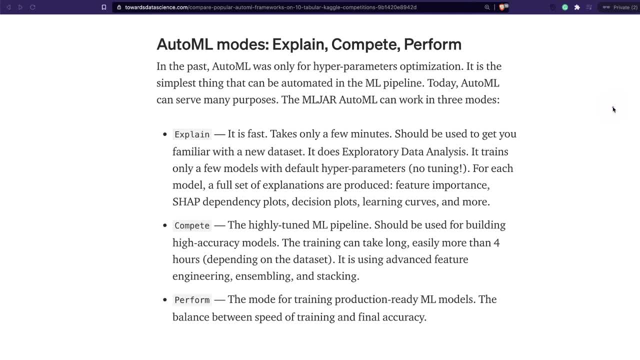 um, a lot of data science projects usually start with pocs and i don't want my team to work, you know, weeks in creating a, creating, uh, a nearly good model, not maybe the best nearly good model, uh and uh if. if that is the case, i would probably, you know, fall back to auto ml model and then ask: 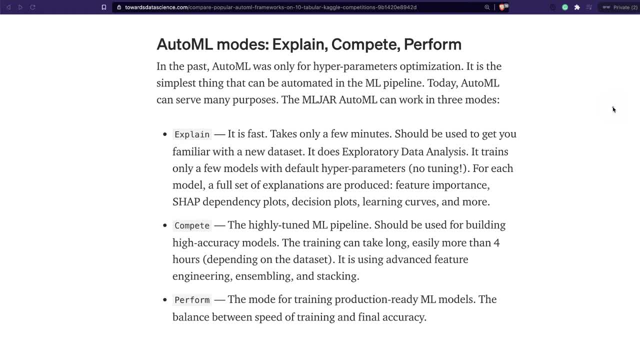 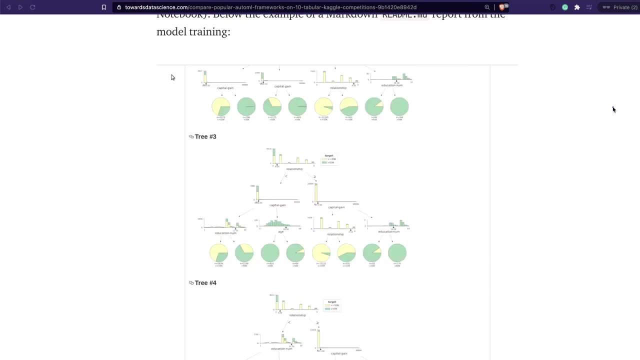 them like: ask my team to use an auto ml framework, build a model, pitch it to my um or responses and then, you know, win the project and then move forward. so these are some reasons why i- i i at least- would use auto ml, because i strongly believe that data science, data scientist. 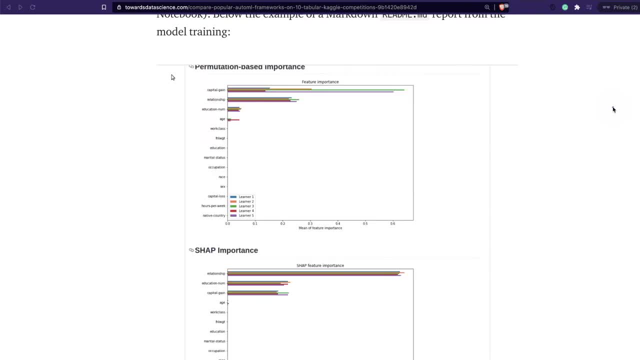 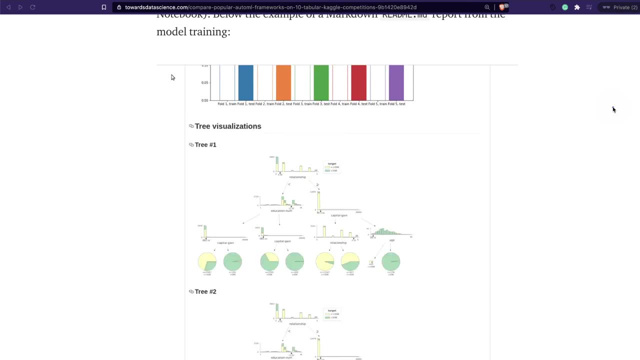 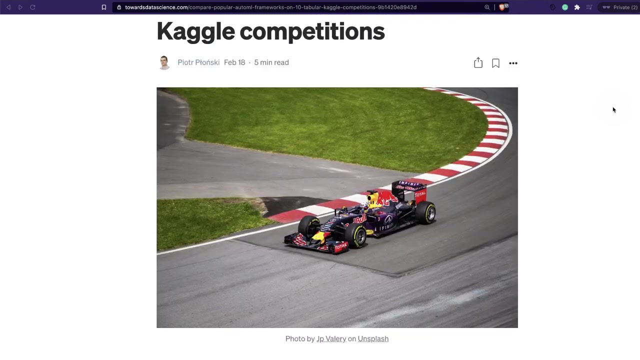 time is well spent in solving the problem, the actual problem, rather than, you know, spending time and creating 10 different models or 20 different models or 30 different model. if your job requires you to do that thing, that is fine, but in most cases, i think this is this- is effective. and one final call out about ml jar. so, according to this author, 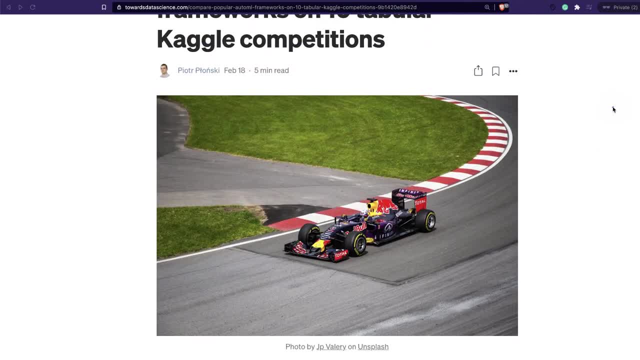 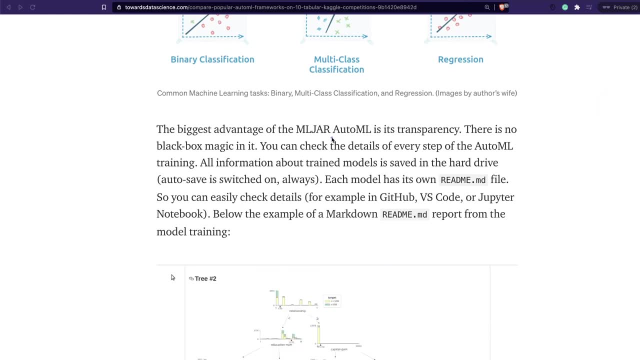 um, who is also, you know, like i said, the creator of ml jar, peter blonsky. ml jar is ml jar is more transparent. so a lot of auto ml models, if you see, the problem is you actually do not know what is happening behind the scene. there are a couple of, you know, like libraries, for example, if you take h2o. 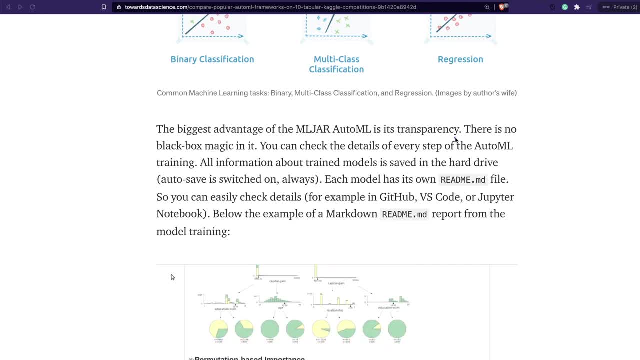 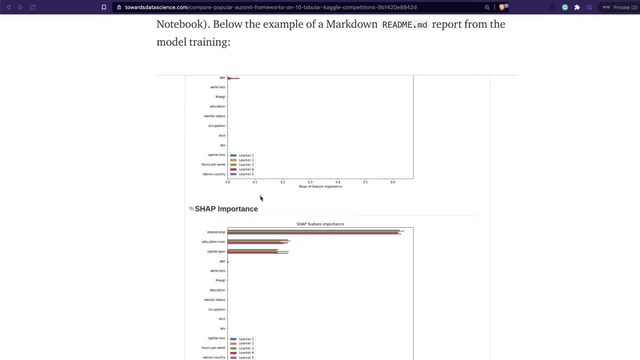 as a. as an example, i have seen uh h2o giving very good, detailed information about the model that is um that is being built, uh and ml jazz, which is that. so biggest advantage of ml jars auto ml framework is its transparency, like you can even see in this animation that you you get to see. 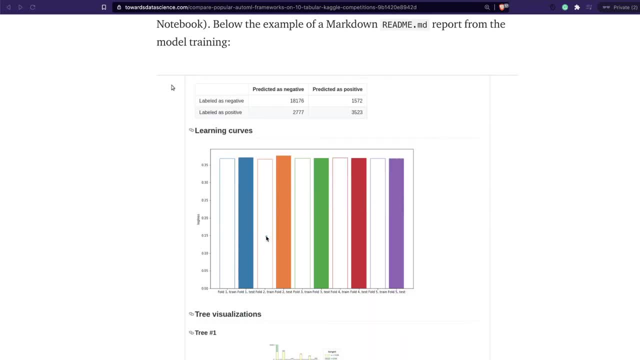 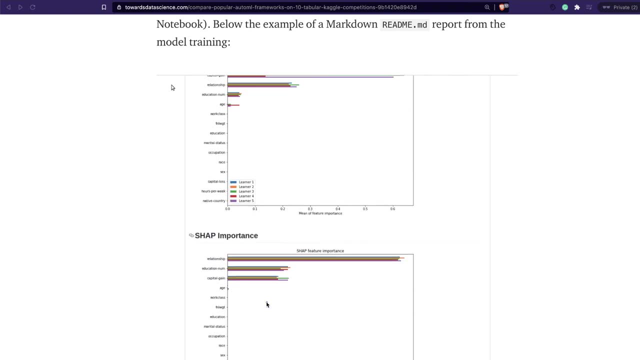 sharp importance, which is some sharp. uh is a is a way to interpret your model and then you can also see, then it is building your graph and then this is quite easy for you to explain to your business about what is happening, uh, why a particular variable is important, why a particular variable. 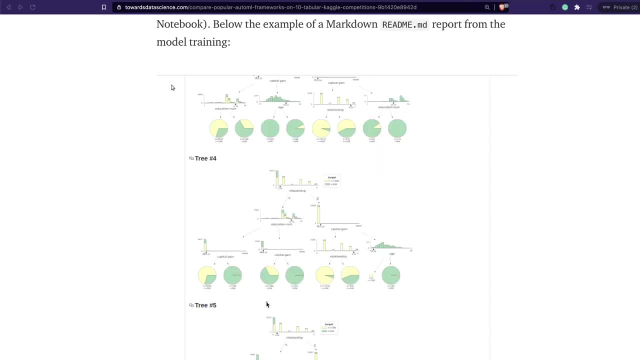 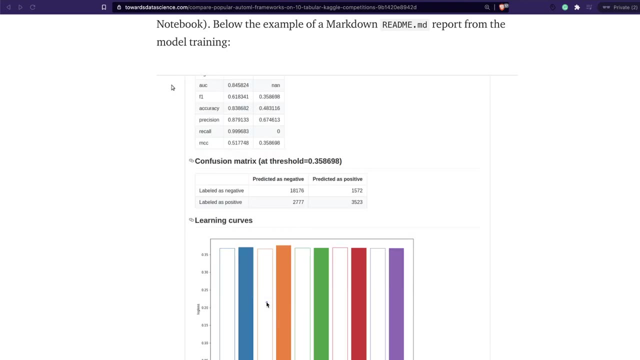 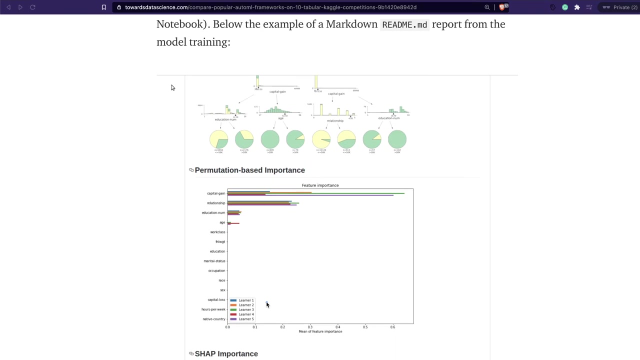 is not important. rather than just reporting the evaluation metric, this could also mean that, um you, you are doing a job that business people can connect with, so that way, ml jar looks again like an exciting prospect. i would probably try out ml jar uh soon, either on a kaggle competition or a. 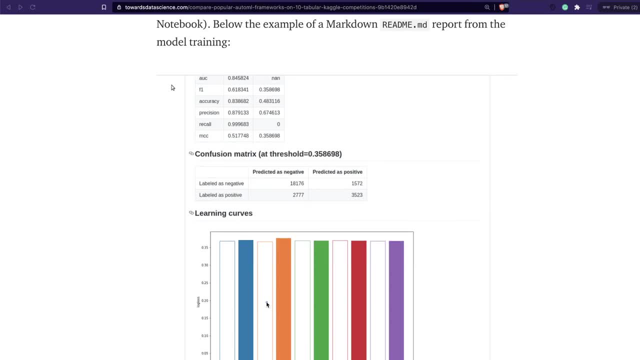 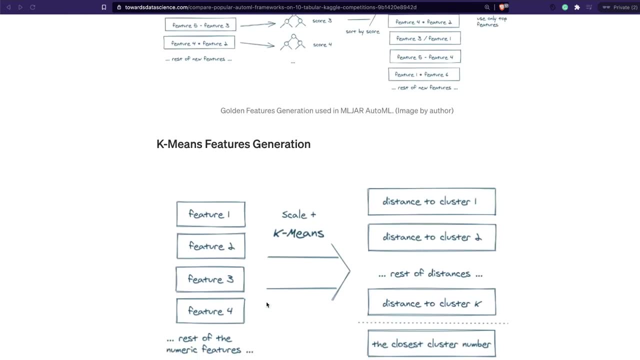 or a just on a data set, and then i would try to make a video out of it and then share it with you, and i hope that this video has been helpful to you. so, if you have used auto ml packages, i think this is high time for you to try out auto ml packages. uh, auto ml packages are really awesome. 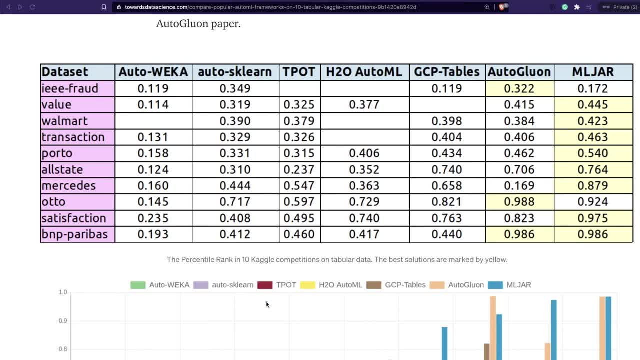 and, uh, you should, you should really, you should really. you know, try your um, um luck with an auto ml packages and see how it works out, um, especially in an organization setup, how it is being received, or all those things. i hope this video was helpful to you in um getting started with auto ml um or at. 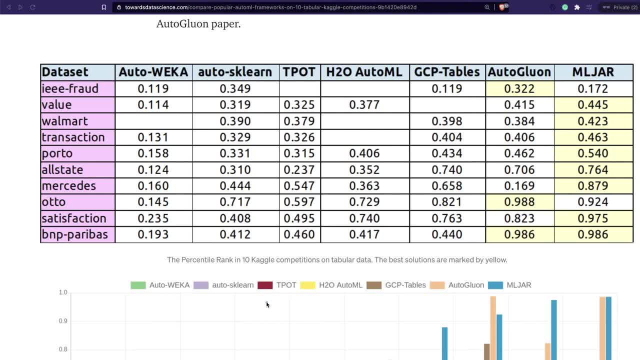 least you know to know about auto ml, and then to which video i have uploaded it for you. so i hope you enjoyed this video and i will see you in the next one. bye, bye, bye. auto ml library that you should be, you know, using more frequently. or, if you want to start with the 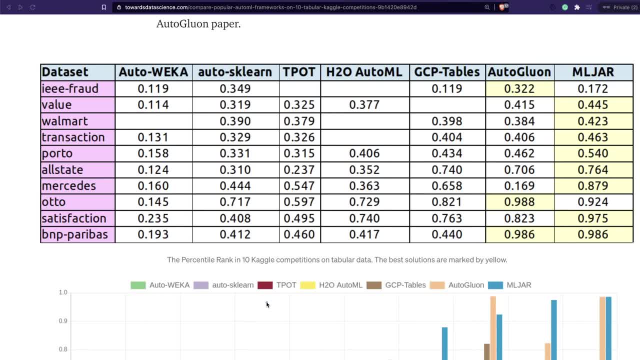 baseline model, auto glue on and ml jar are the leading contenders according to this table, but also there are a lot of other auto ml packages that that is left out. um, in this analysis, pi carat is a very popular package these days. um auto keras is another popular package. there are a lot. 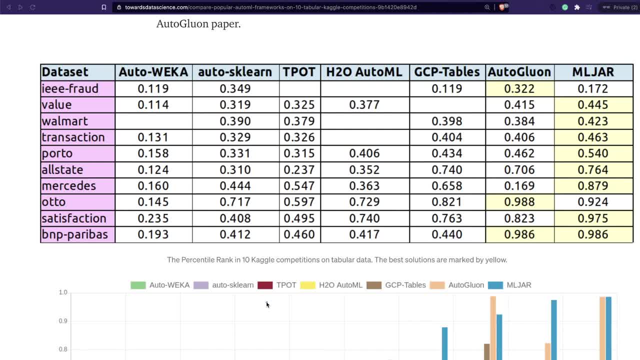 of other packages like this. that is not part of this analysis, but according to this analysis, these auto glow and animals are to good framework. you should definitely check it out then see the performance of auto ml packages. thank you so much for listening to me and uh, thanks, uh, thanks to.